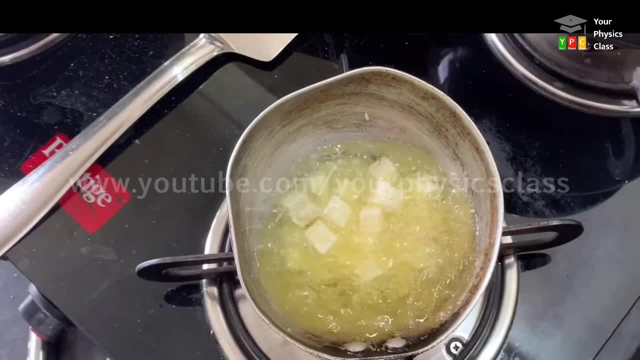 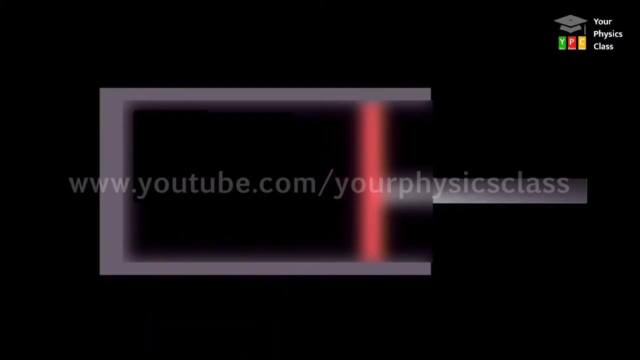 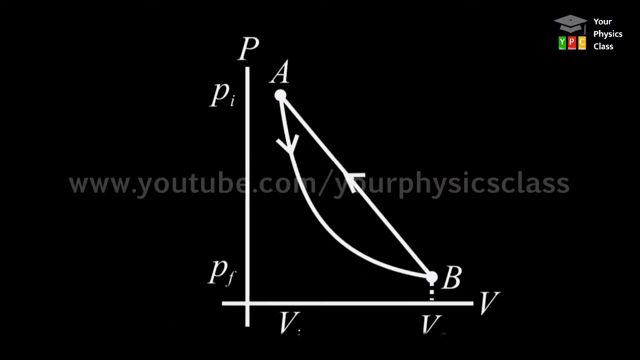 no loss in energy, but a real thermodynamic process will always encounter some loss due to friction or some other dissipative forces. The PV diagram for irreversible process is shown on your screen Area under the path. A to B and B to A are different, showing energy loss in the process. 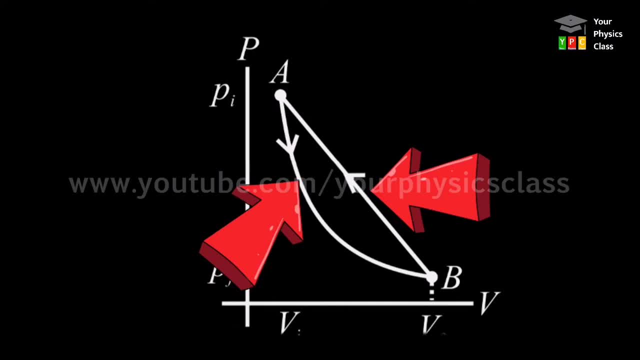 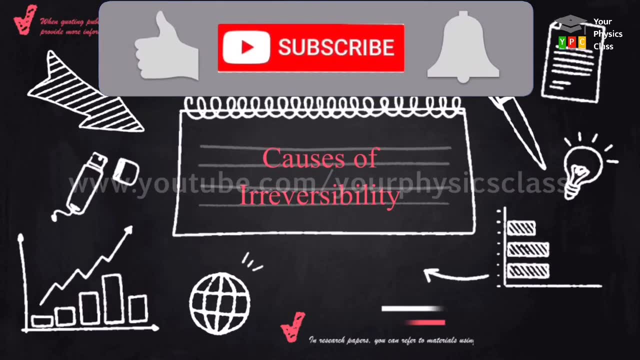 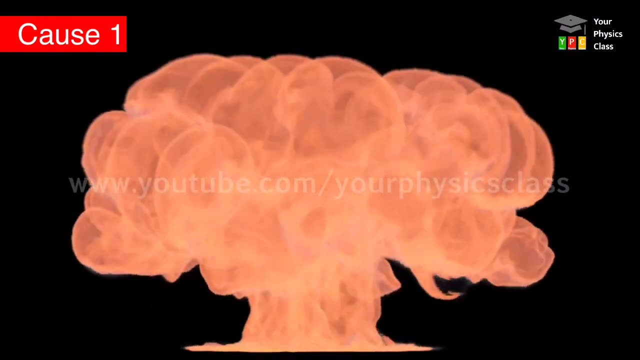 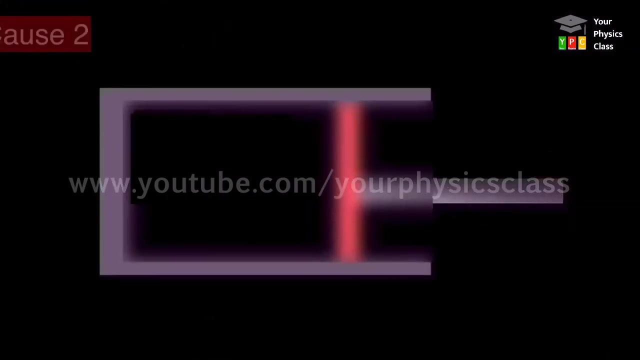 Different paths indicates that system do not retrace same path when the process is reversed. Let us now see causes of irreversibility. Many processes, such as free expansion or an explosive chemical reaction, takes the system to non-equilibrium state. and the second cause is most processes involves 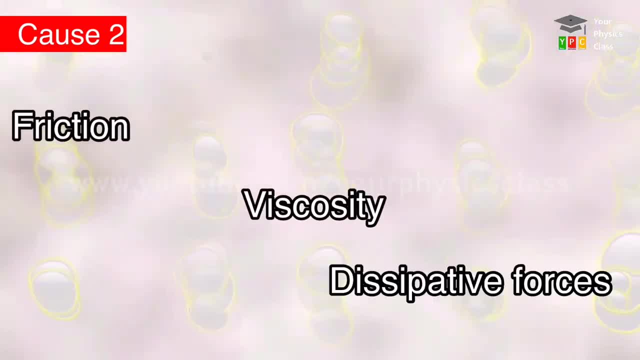 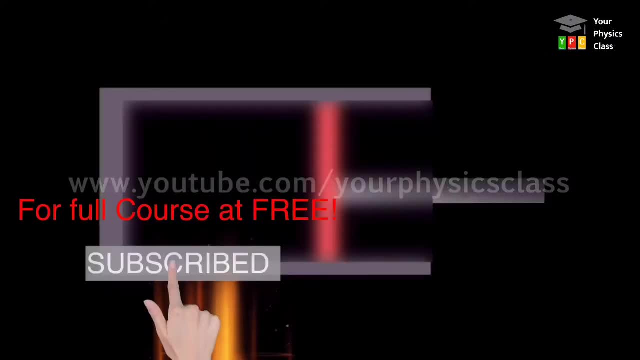 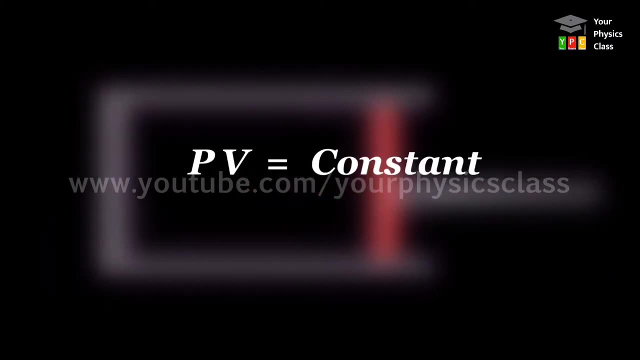 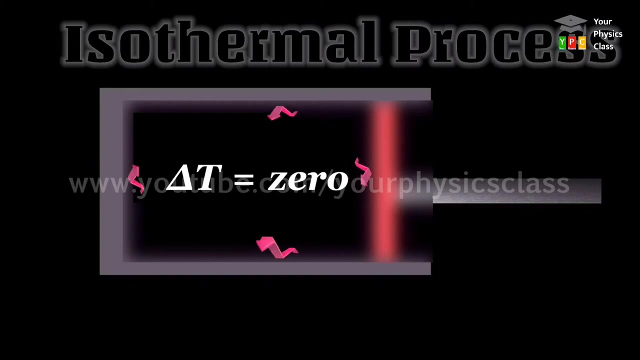 friction, viscosity and some other dissipative forces. Second is isothermal process. The process in which change in pressure and volume takes place at constant temperature is called isothermal process. In this process, changes are extremely slow, so that thermal equilibrium with surrounding is maintained throughout the 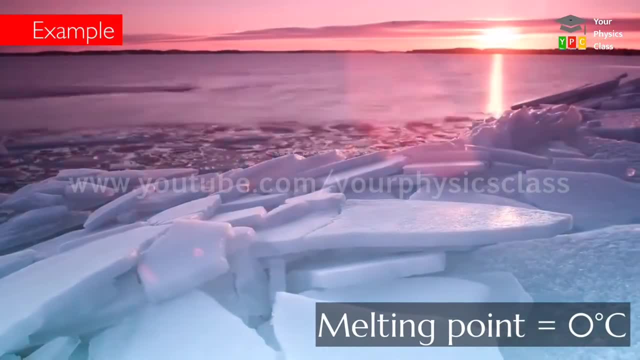 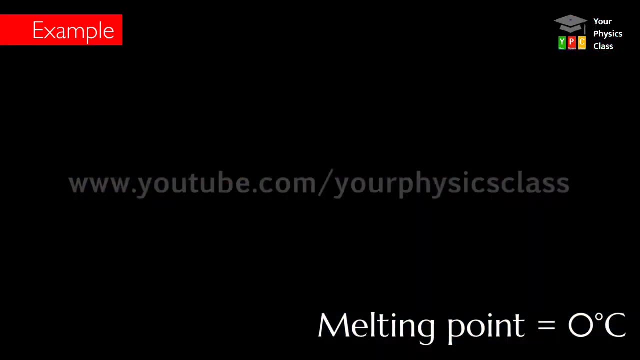 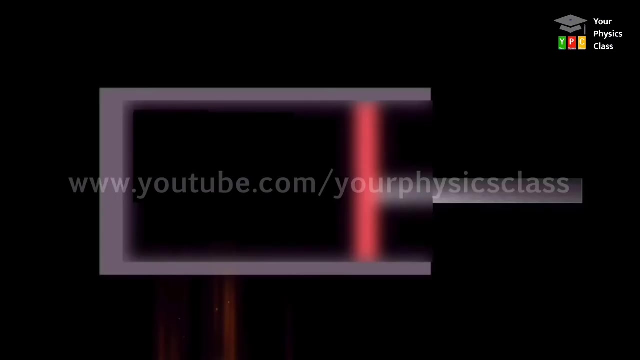 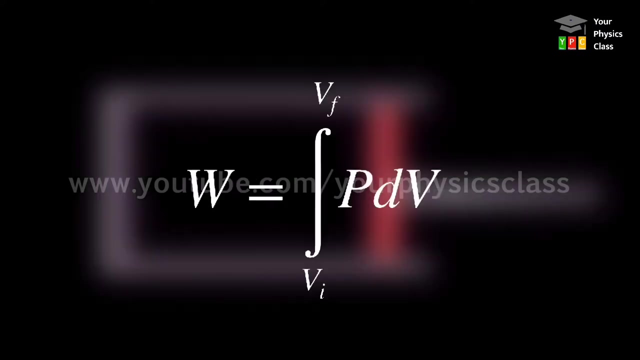 process, For example melting of ice, takes place at constant temperature, Hence it is a isothermal process. Thermodynamics of isothermal process During isothermal expansion from VI to VF. work done to bring the expansion is W equals integration VI to VF of P into. 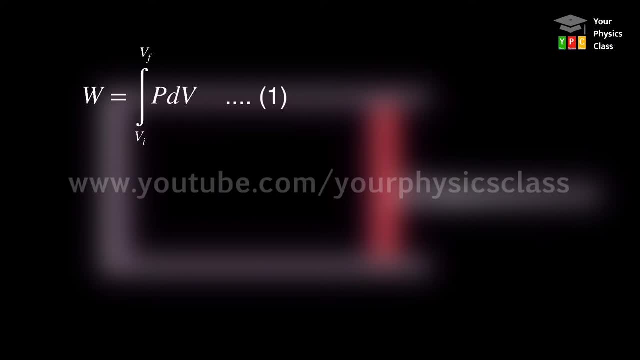 dV. Let us call this equation as number one For ideal gas PV equal to NRT. in usual notations, This implies that P equals NRT by V. Substituting this value in above equation number one, we get W equals integration between: 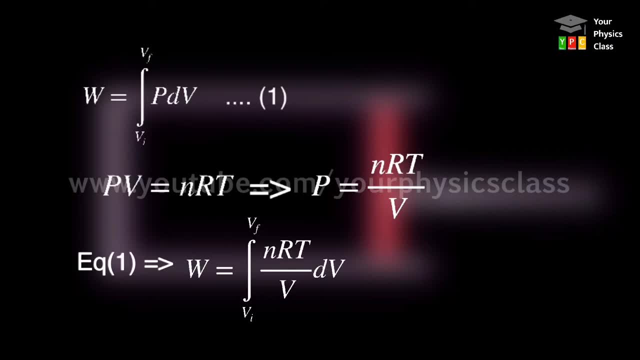 the limit VI to VF of NRT by V into dV. Therefore W equals NRT times natural log of VF upon VI. So you have to remember this step. those who don't have mathematics, So your mathematics details involving these steps are not mentioned, So direct. 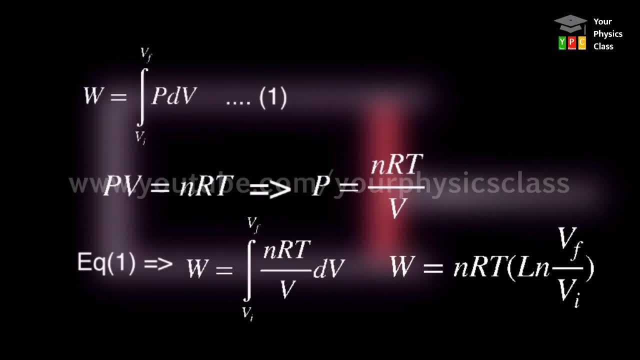 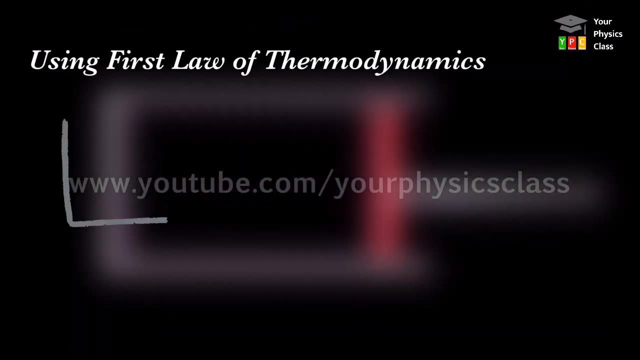 result is expected here? Okay, and it is good for the sociology and fishery students. That means the student, those who have not taken mathematics at twelve standard. for them, this step will be easy to remember Now. using first law of thermodynamics, Heat supplied is equal to. 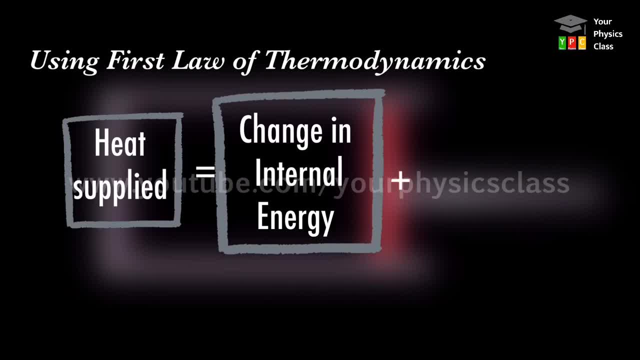 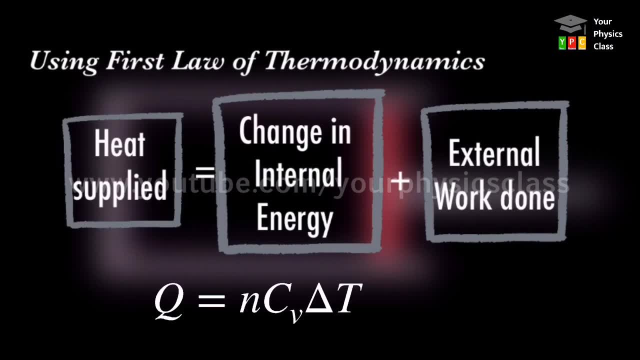 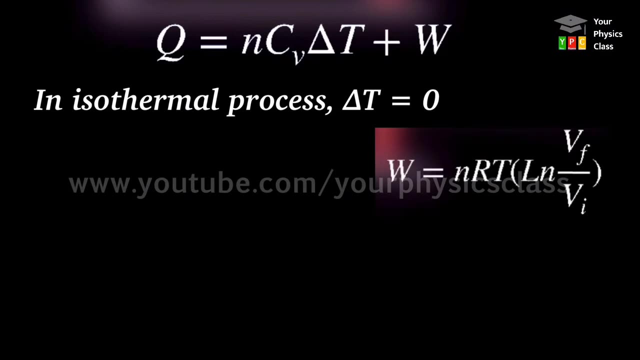 change in internal energy plus external work done in the expansion. So we can write this as: Q equals N times CV, delta T plus W. Therefore Q equals zero plus NRT. natural log of VF upon VI. Here change in temperature is zero, since the process is isothermal. 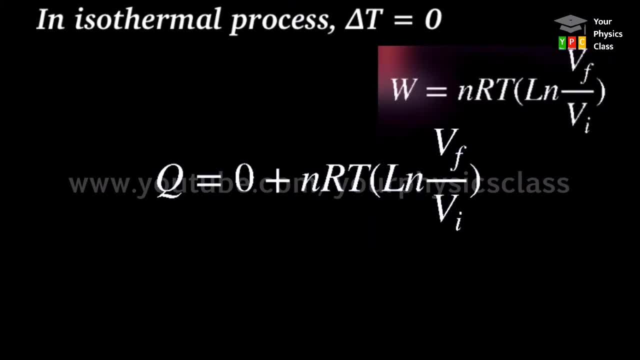 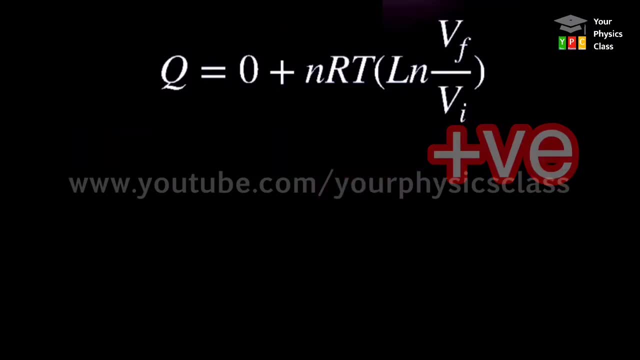 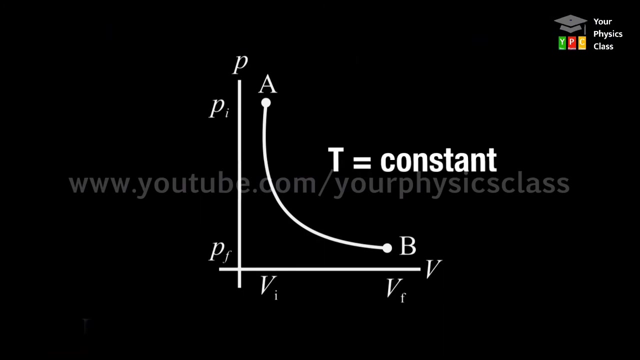 That is why the first term becomes zero. When gas expands, VF becomes greater than VI. Then system does positive work and does negative work. when gas compresses, that is, VF is less than VI. Any change of phase occurs at constant temperature is called isothermal process. 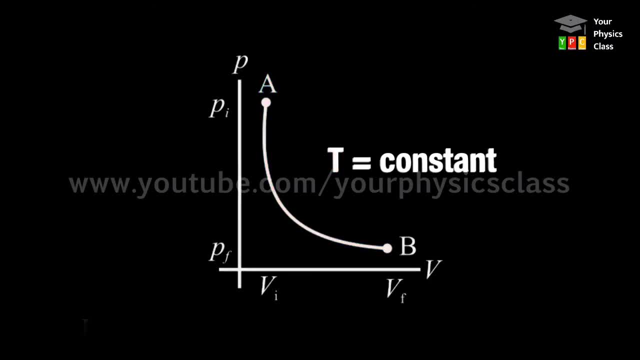 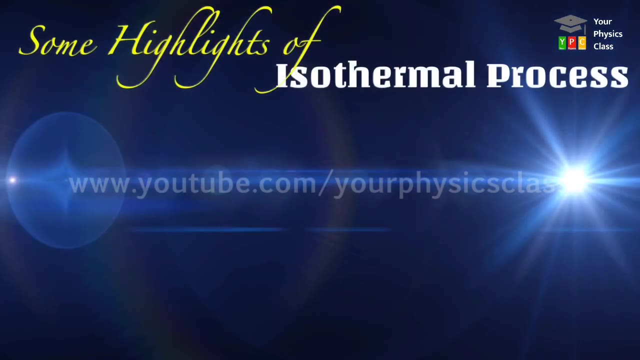 The PV diagram of an isothermal process is shown on your screen. It is called isotherm Since the process occurs at constant temperature. Let us revise the isothermal process. In this process, equation of state is: PV equals constant. The temperature change is zero throughout the process. 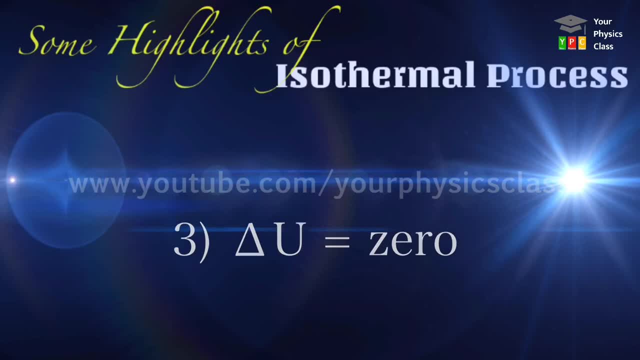 The change in internal energy is also therefore zero. The heat supplied is used for work done. External work done is nothing but the product of constant pressure and change in volume. An isothermal change is a very slow change. The system exchanges heat with its surrounding and is in thermal equilibrium. 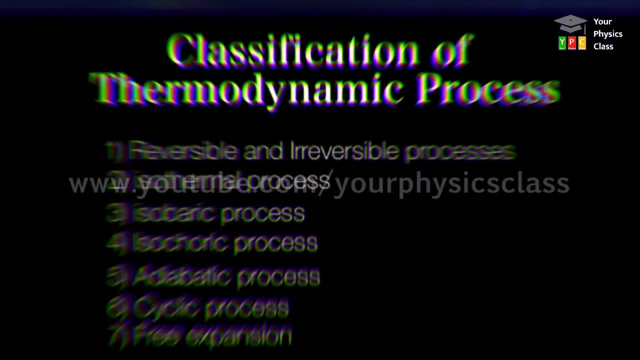 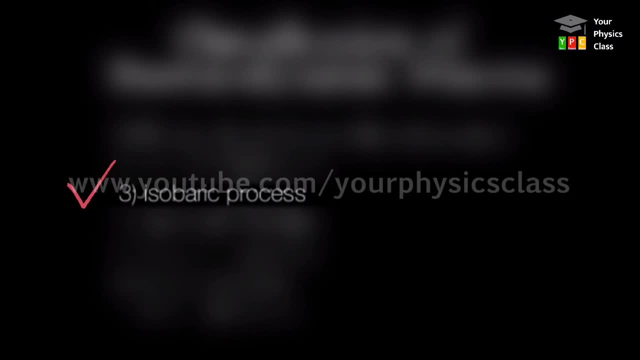 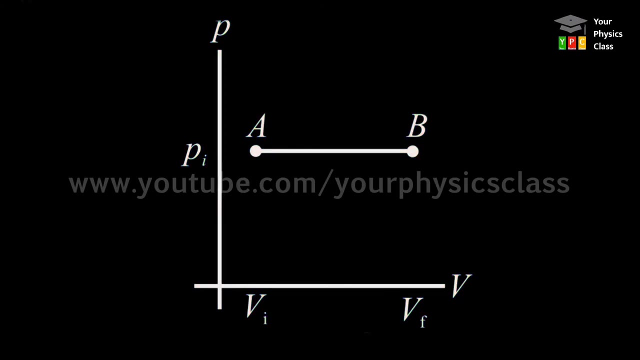 with it throughout the change. The thermodynamic process that takes place at constant pressure is called as isobaric process. The PV diagram for this process is shown on your screen. Since the pressure is constant in this process, therefore, the PV diagram is called isobars. 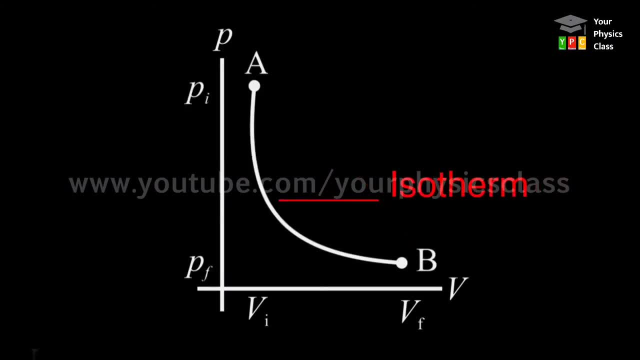 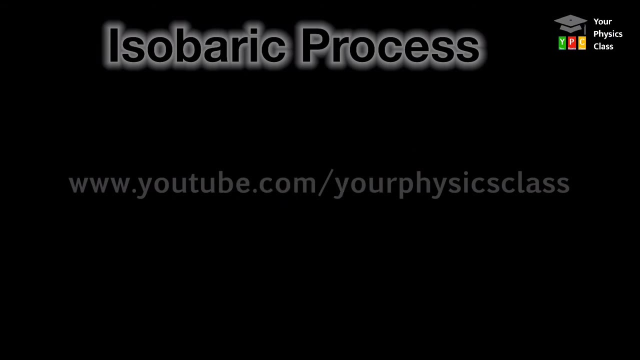 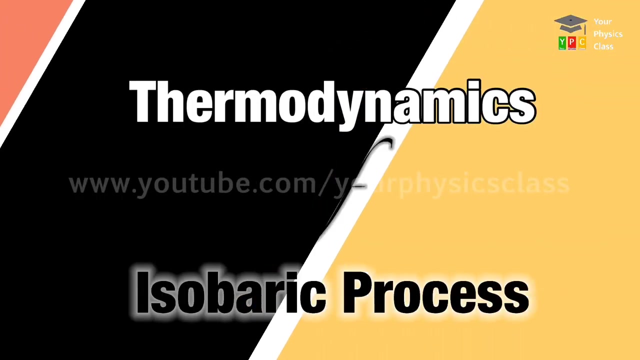 Remember, in isothermal you called this diagram as isotherm because temperature was constant. Now pressure is constant. therefore we call it as isobars For an isobaric process. change in internal energy, the heat supplied and the work done by the system can never be zero. Now let us discuss thermodynamics. 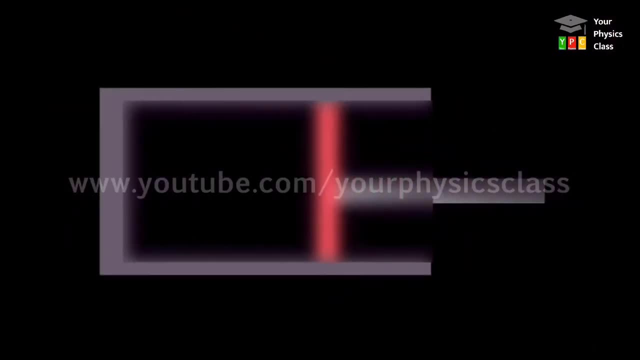 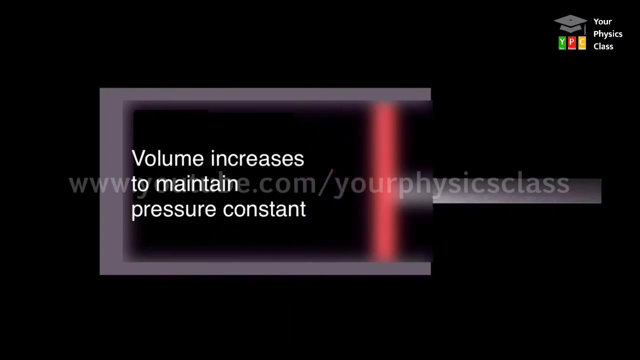 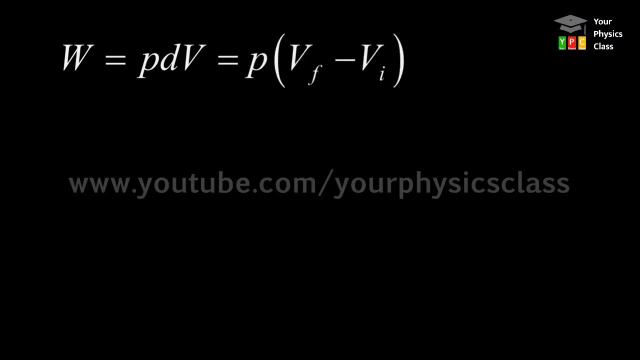 of isobaric process. The system undergoing isobaric expansion is shown on your screen. The work done during isobaric process is given by: W equals P times G and G equals T- inverse delta- delta times of G. The next equation us to learn is slope arrays that use the internal energy of the system at constant volume is given off. 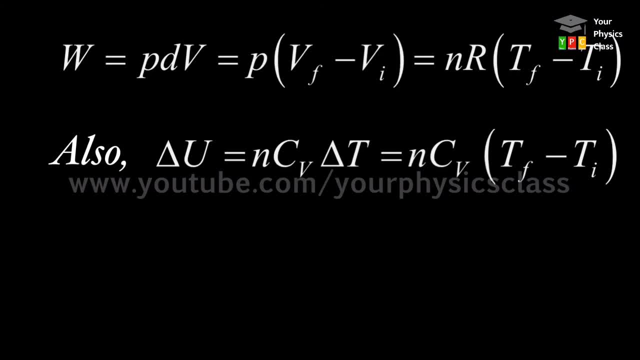 But we must not forget that if we are not able to solve a corresponding problem as we do, we need to find an extra output and solve this by its form of combustion, because costing物 방, to demand delta U equals n times Cv, delta T. 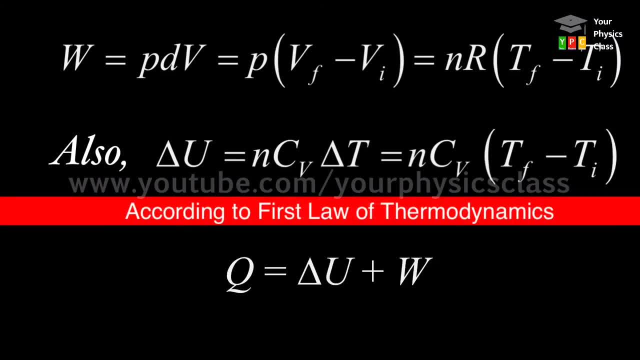 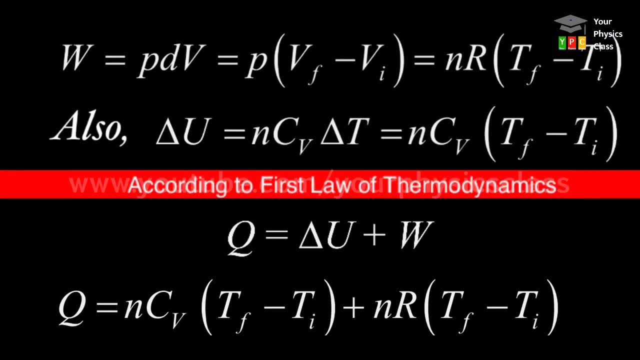 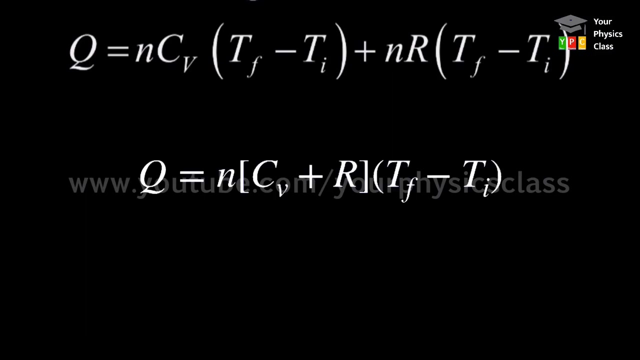 Now, in accordance with first law of thermodynamics, we may write: Q equals nCv times change in temperature plus nR times change in temperature. Here the term change in temperature and number of moles, Cn. both are constant, thus taken common. So the equation takes the form: 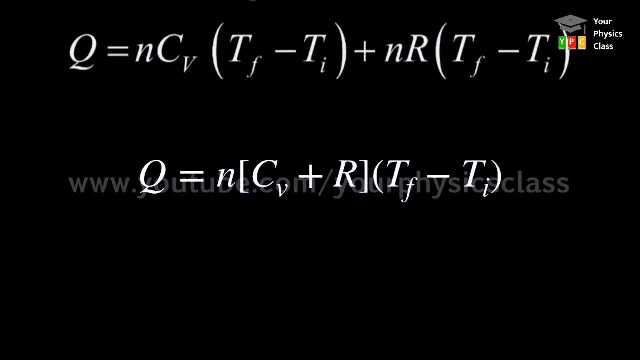 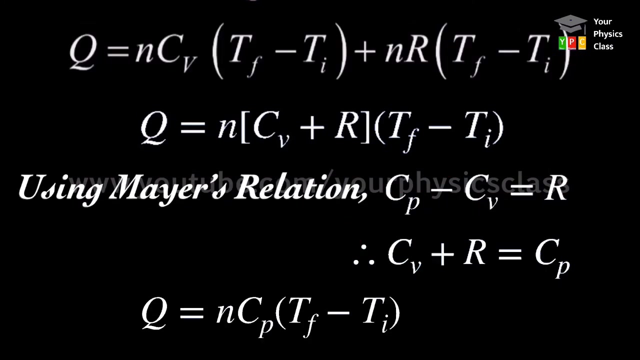 Q equals n times Cv plus R into Tf minus Ti. Using Merz relation, Cp minus Cv equals R. we get the value of Cv plus R which is equal to Cp, that is, specific heat at constant pressure. So the equation becomes: Q equals n times Cp into change in temperature.